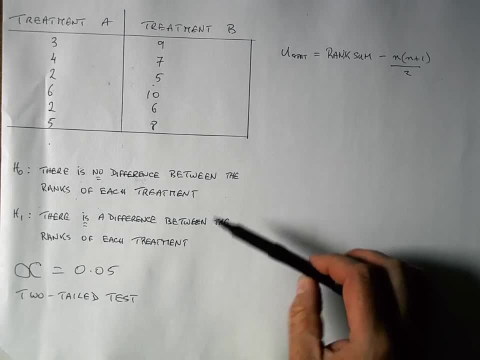 rank based test and our alternative or research hypothesis is that there is a difference between the ranks of each treatment. So in other words, I'm saying in my null hypothesis is that the both treatments are the same and in my research alternative hypothesis that the treatments are not the same. 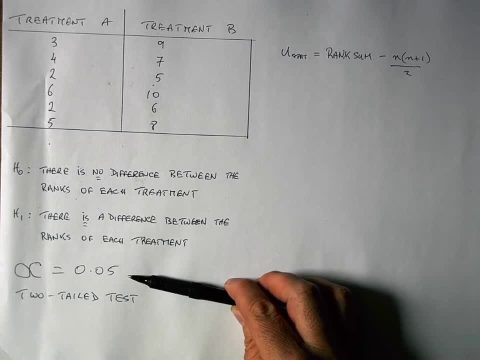 same. We're going to test here at an alpha value of 0.05, and we haven't indicated a direction for our test, so we're going to have a two-tailed test in this case here. So it's a two-tailed. 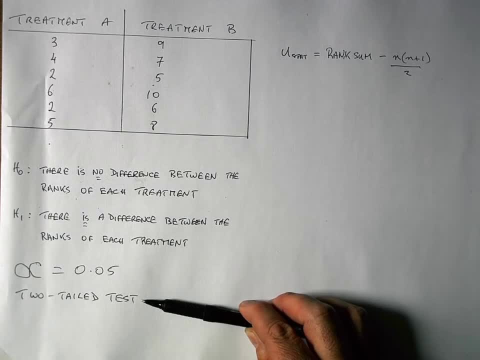 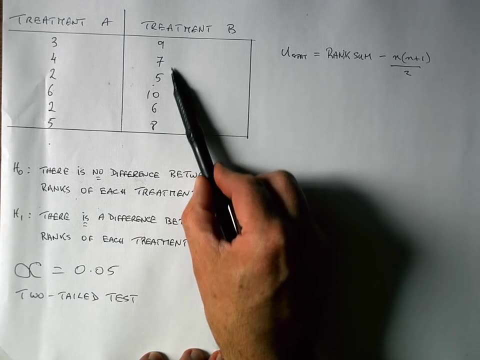 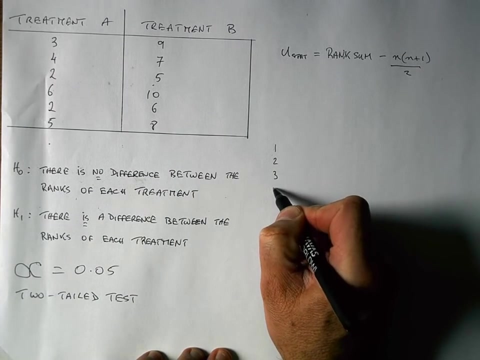 unpaired or independent Mann-Whitney test. So as it is a rank-based test, I need to be able to rank all of these numbers: my six values for treatment A and my six values for treatment B. So that gives me a total of 12 numbers. So my first task is to rank each of these 12 values from 1 to 12.. So I'm 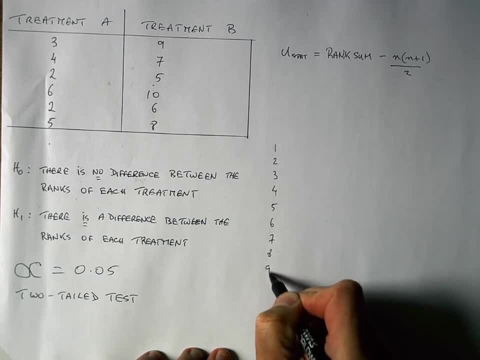 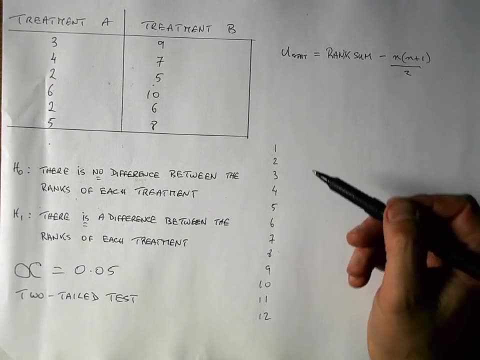 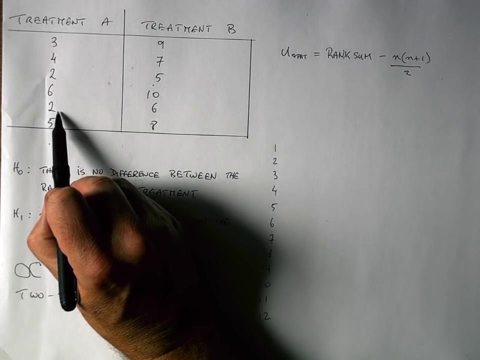 going to write out just a series of numbers, from 1 to 12, so that I can rank each of my individual values here. So now I'm going to rank all my values from the smallest to the largest values. I'm going to look for the lowest value to rank it as number 1.. I can see I have a 2 on my data and I also 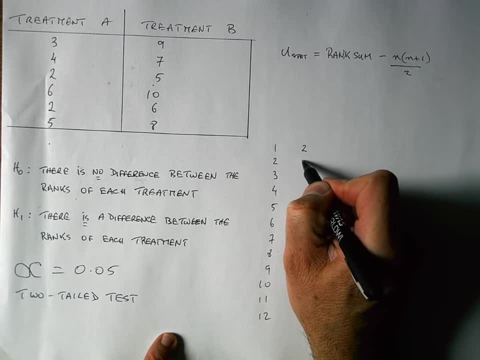 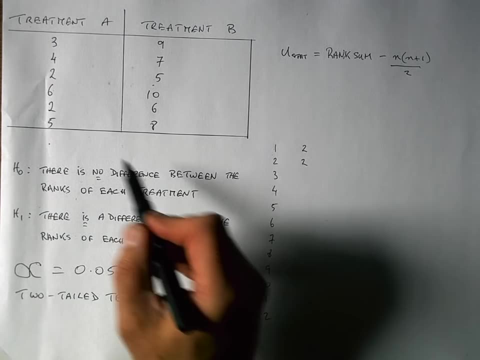 have another 2,, so I can rank my first 2 as number 1 and my second 2 as number 2.. Now that gives us a tie, so we'll have to come back to that in a few moments. My next highest value is 3, so 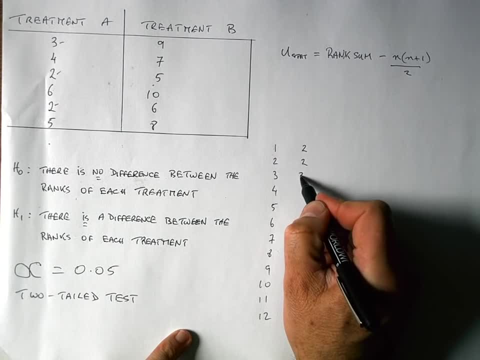 as a result of that, I'm going to rank my first 2 as number 1 and my second 2 as number 2.. As I'm going along here, I'm going to tick off each of the values to indicate that I've scored them. 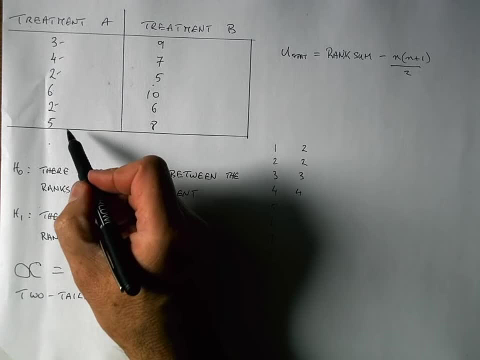 Number 4 is my next highest value, and then when I come to the next highest value, which is a 5, so I've got a 5 in treatment A and I've also got a 5 in treatment B, so I've got to put down two. 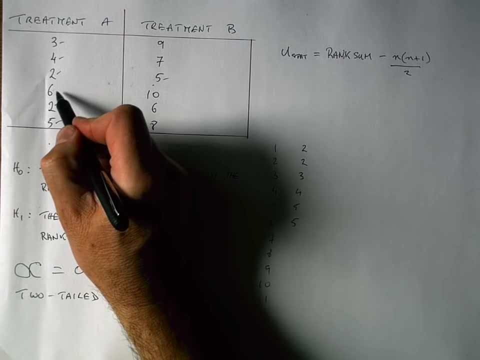 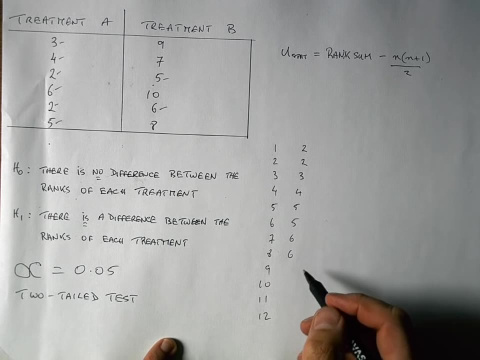 5s here, which is another tie. My next highest value is a 6 in treatment A, and there's also a 6 in treatment B, so I'm going to put down the two 6s here for another tie. Then my next highest. 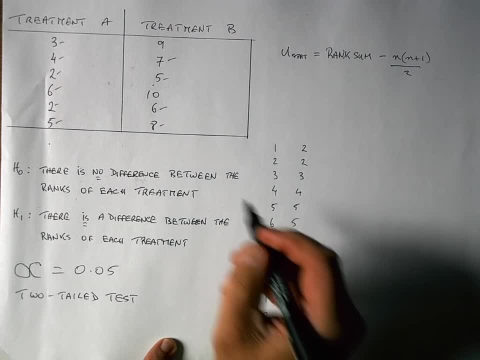 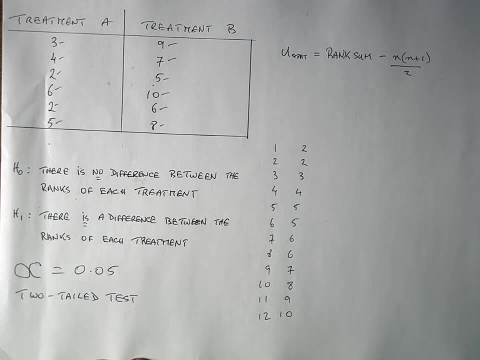 value is a 7.. After that, I've got an 8,, which I'm going to rank as 10.. I've got a 9,, ranked as 11, and finally I have a value of 10,, which is my highest value, ranked at 12 in this case, here Now before. 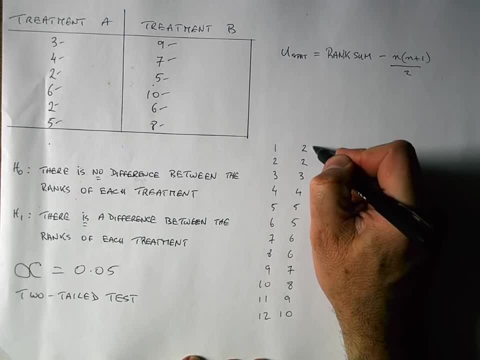 we do any calculations, we have to check for ties and, yes, we have some ties here. We have two 2s, we have two 5s and we have two 6s, So we need to be able to rank those. We can't use a ranking of. 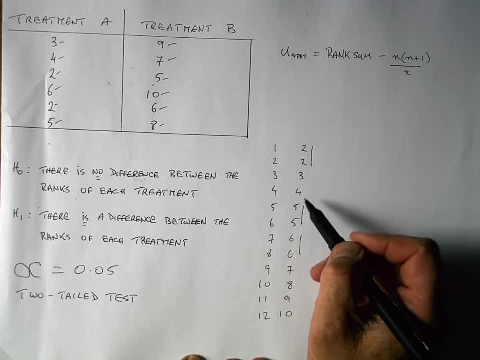 1 and 2 here, because we don't know which 2 it is. So, for example, where we have two values of 5,, 1 is in treatment A and 1 is in treatment B. we can't use a ranking of 1 and 2 here, because we don't know which 2 it is. 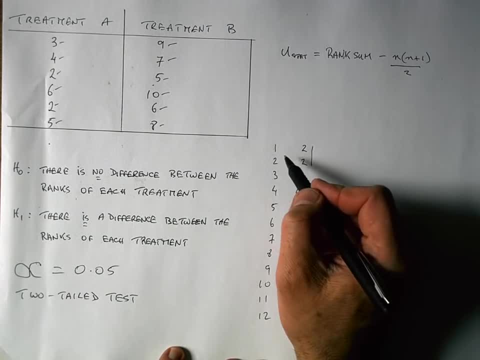 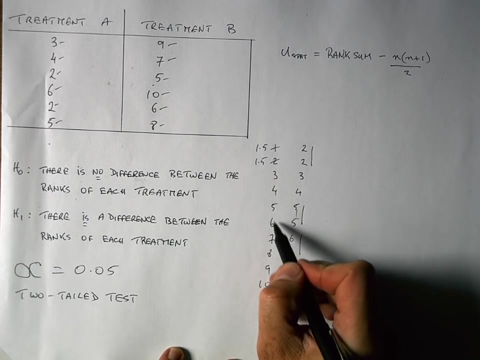 So we need to rank those equally. So the way to do that is we just take the average of the rankings. If we have two values, just add the two values together and divide by 2.. So 1 plus 2 is 3, divided by 2 is 1.5.. So my new rankings here are 1.5. Go down to my two 5s which are ranked. 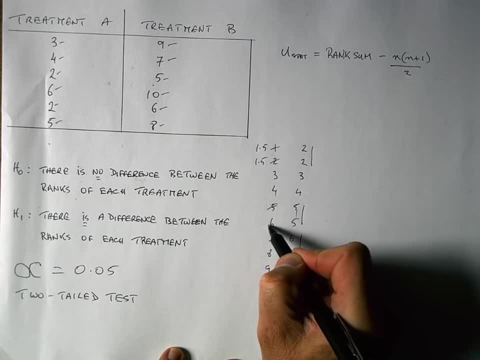 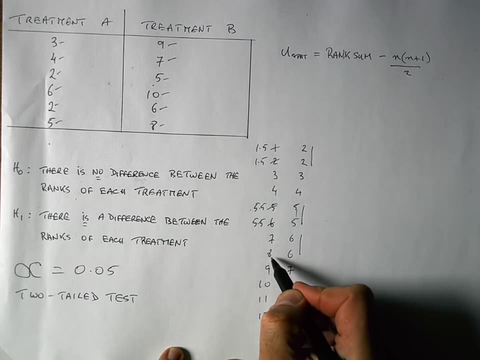 5 and 6.. So 5 plus 6 is 11, divided by 2 is 5.5.. My final rankings here: take the rankings 7 and 8, add them together and divide by 2.. So 7 and 8 is 15,. 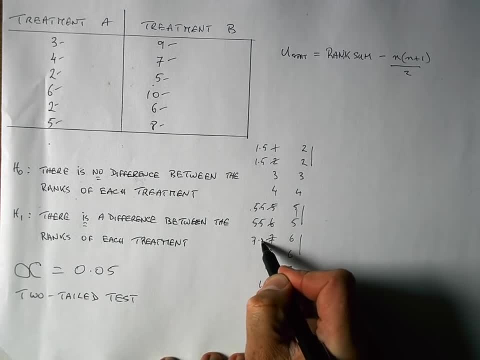 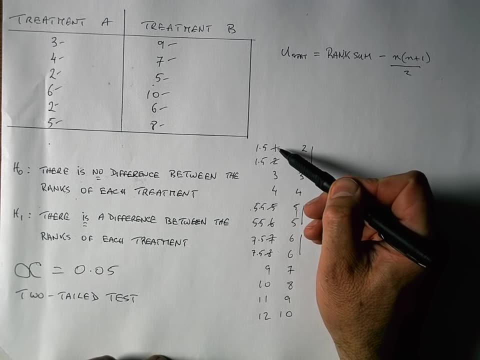 so to divide that by 2 gives us rankings here of 7.5.. So that's how we deal with ties. So now we can see in our data: for example here we've nothing ranking as ranking number 1, and we've nothing ranking as ranking. 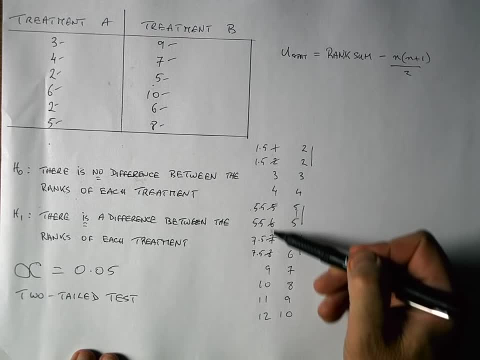 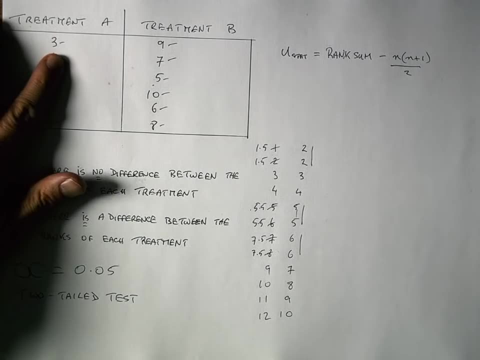 number 2, and so on. So now I want to take these rankings here which I've just worked out and put them beside each of the scores over here in our left-hand side. So for example, in treatment A, the value of 3, we can see over here that. 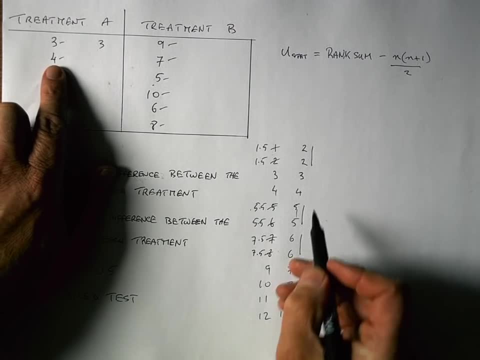 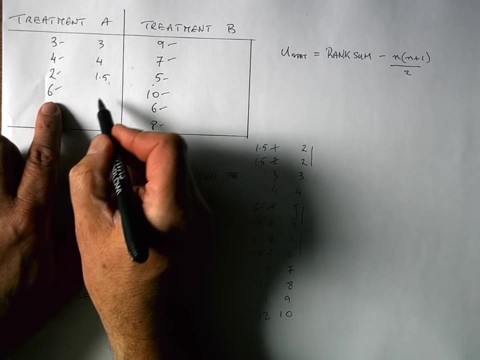 that ranked as the third highest value, the value of 4 ranked as the fourth highest value. Then I come to a 2, which was ranked as 1.5.. Let's put that in there. And I come to 6,, which was ranked as 7.5.. 2 was ranked at 1.5. 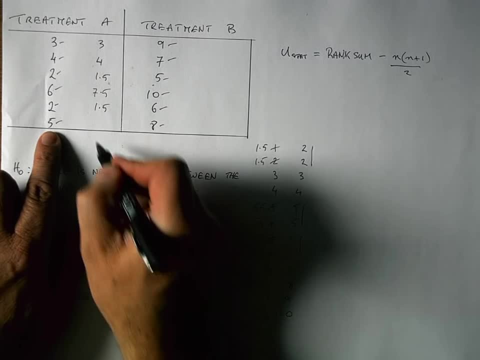 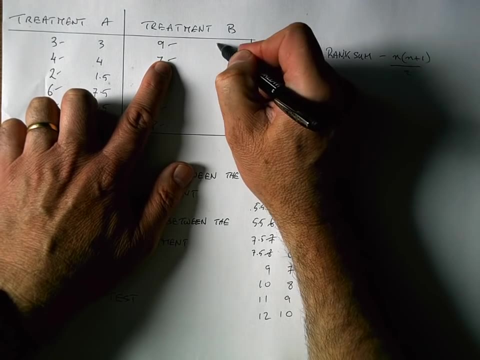 again, And 5,, as we can see, was ranked at 5.5.. Over to treatment B, we can see that 9 was ranked as 11.. 7 was ranked as the ninth highest value. 5 was ranked at 5.5.. 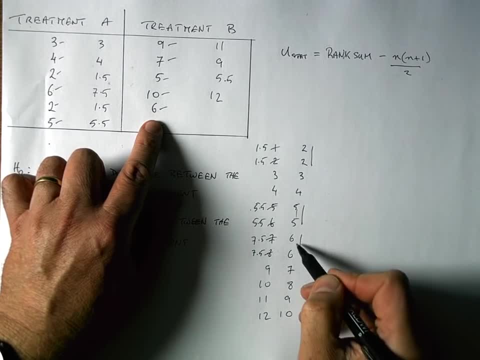 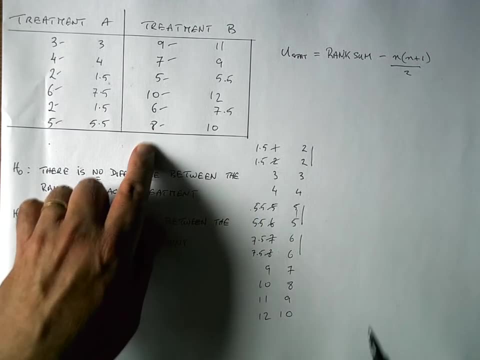 10 was ranked at 12.. 6 was ranked at 7.5, another one of our ties- And our final value, 8 here was ranked as number 10.. So now that we have all the rankings here, our next job. 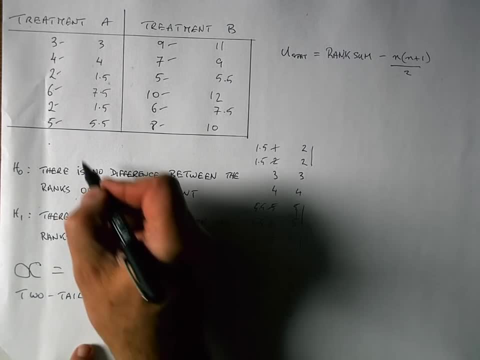 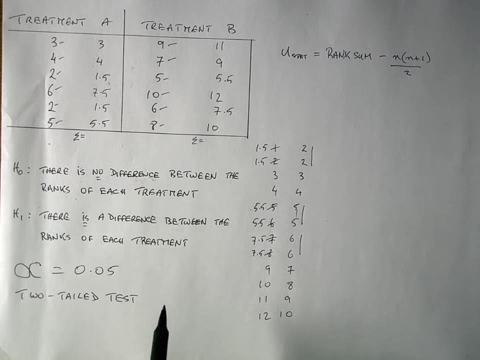 then is to sum all of these ranks, because we need to get a value for our sum of each of these ranks. So I'm going to add up all the values for the treatment A, And when I add all of these up, I get a value of 23.6.. 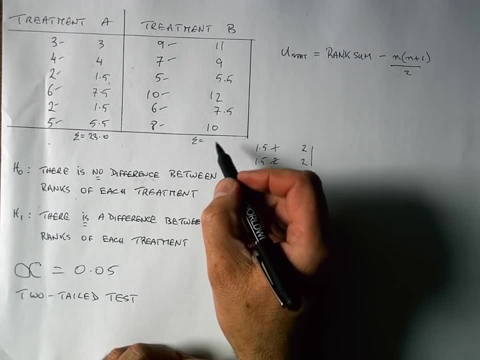 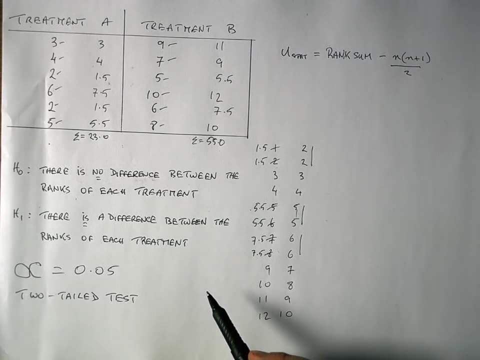 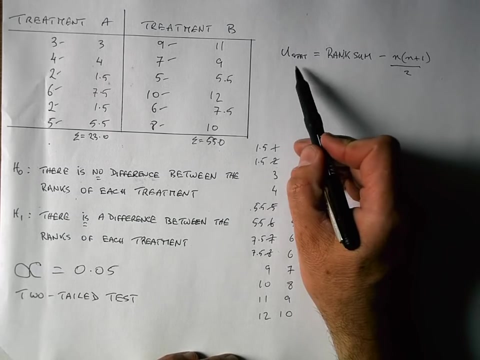 And when I add up all the values for treatment B I get a value of 55.0.. So these are my rank sum for each of the two values. Now I'm ready to actually do the calculation for the U statistic, which is what the Mann-Whitney U test is based on My U statistic here in. 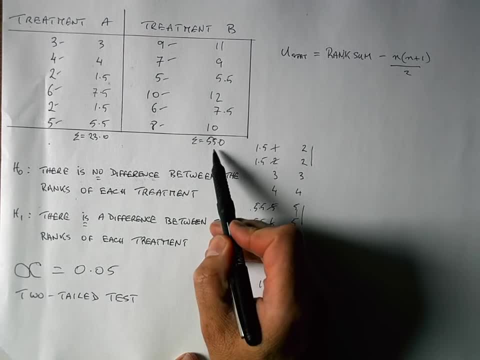 the formula it's equal to my rank sum, and I've just calculated the two rank sums for my two groups minus n, the number of values in each treatment. So that's in my case, here it's going to be 6 for each value. So I'm going to have a 6 here, And I'm going to have a 6 here, and I'm going to have a 4 for each. 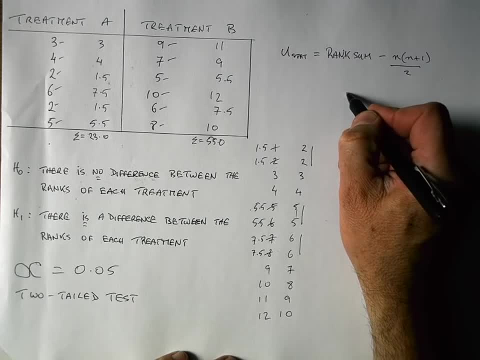 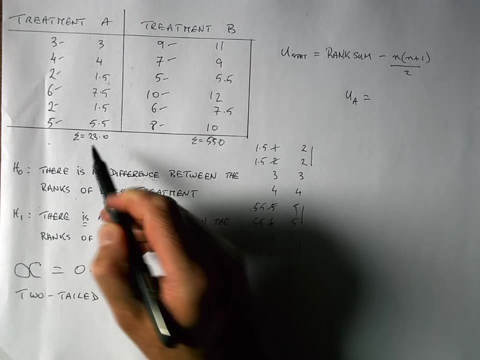 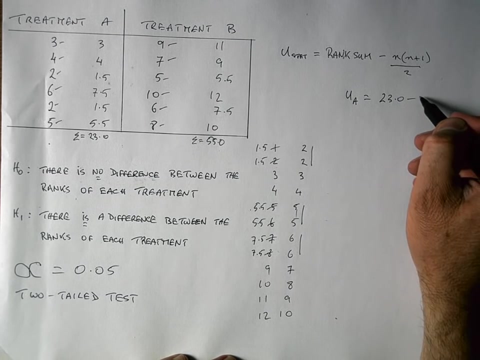 value. so I'm going to have a 6 here and a 6 in here. So let's now work out the U statistic for treatment A. so that's equal to my rank sum value, which is, over here calculated: 23.0, minus n times n plus 1, so I've got 6 values. so that's 6 times 6 plus 1, which 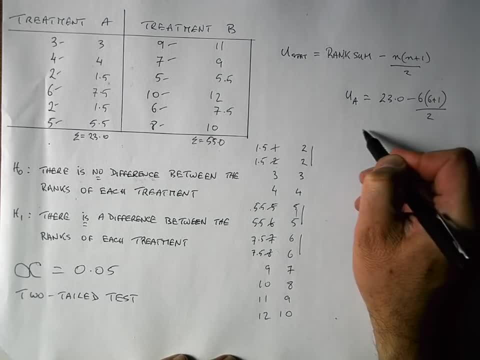 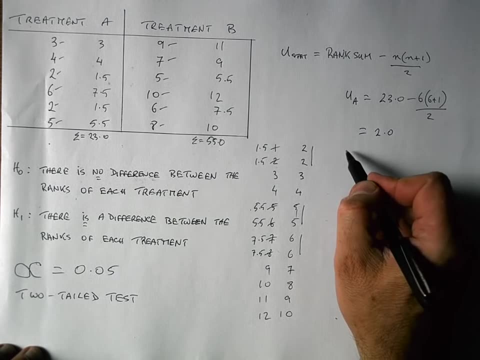 of course, is 7,. divide that result of that by 2, and when I work that out, I get a value of 2.0.. Next now work out the U statistic for treatment B, and that's equal to the rank. 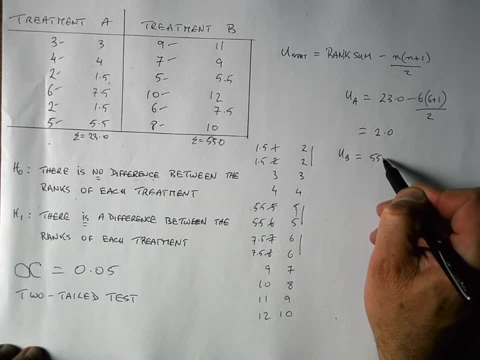 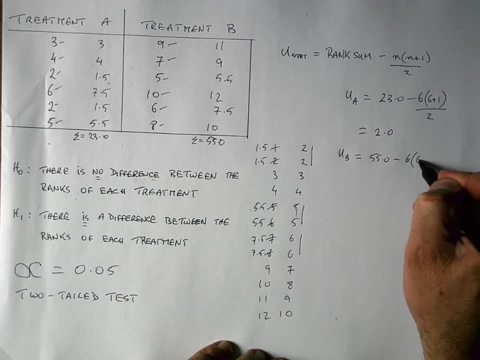 sum, which is 55.0 in this case, minus the n, the number of values in treatment B, which is again 6, times 6 plus 1,. divide that by 2, and when I work out this value here, I: 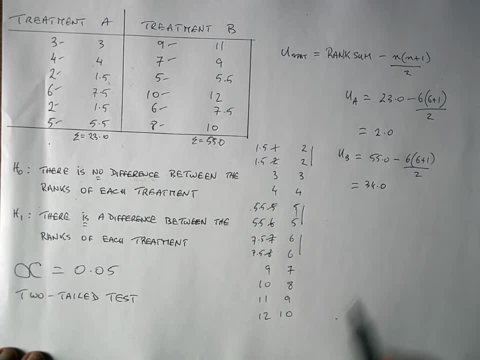 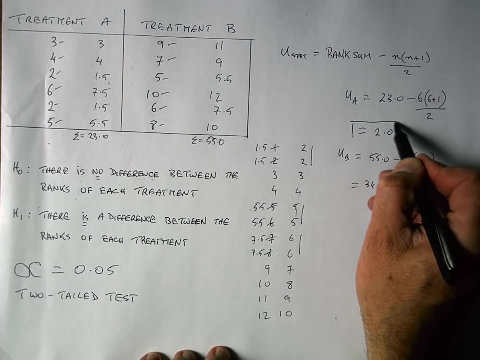 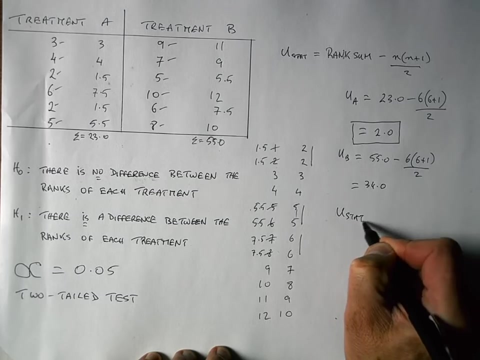 get a result of 34.0.. So I've got two U statistics but I can only use one, and in the bandwidth test the value that you use is the lowest value. so I'm going to use the U statistic for sample A or treatment A, so my U stat is equal to 2.0.. Next I need to determine: 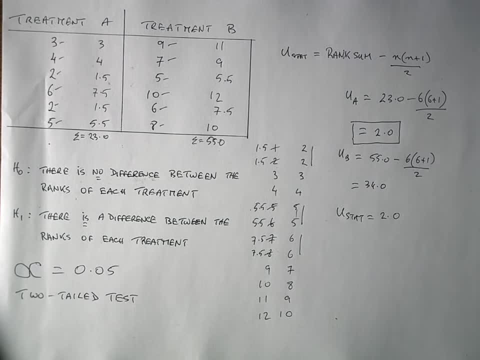 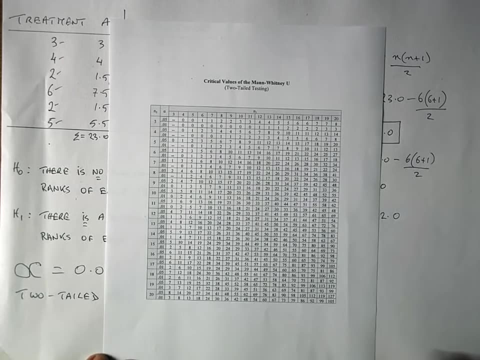 a critical value which helps us accept or reject our null hypothesis. so I'm going to go to a critical value. so the Mann-Whitney U test- and this is for two-tailed testing and it's based on: I need the n1 for the number of values. 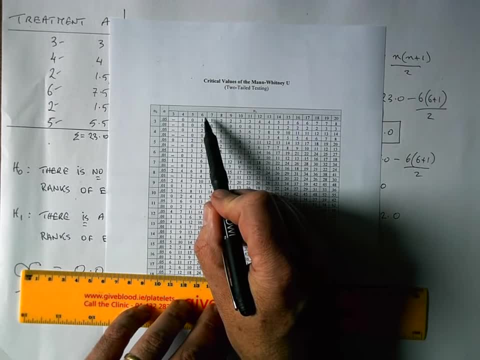 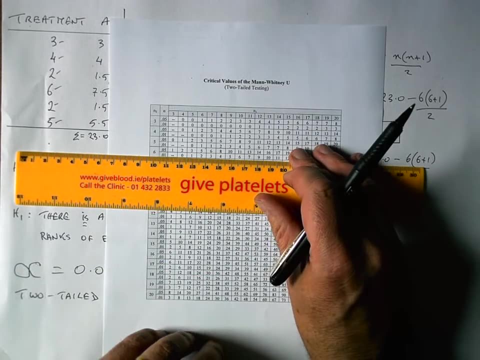 In group 1,, that's treatment A in my case, which is 6, and I also need the number of values in group 2, which is treatment B, which is also 6 in this case. So if I just take the row and where the columns meet, so 6, and column 6 and row 6, here we can see I 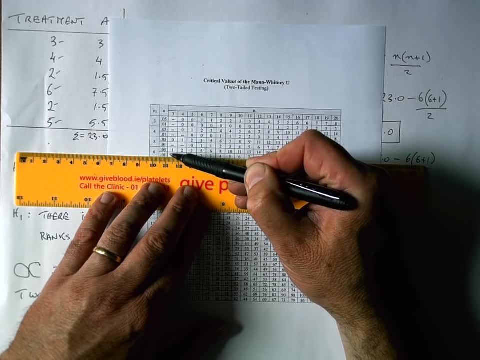 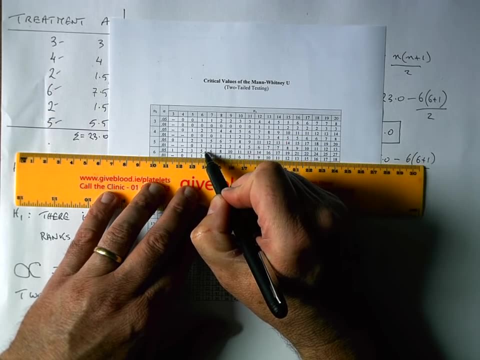 have values for alpha equal to 0.05 and alpha equal to 0.01, and I'm choosing 0.05, and we can see there that the critical value is 5, for n1 equals 6 and n2 equals 5.. So that's. 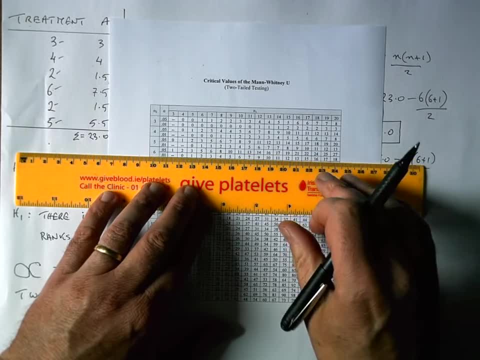 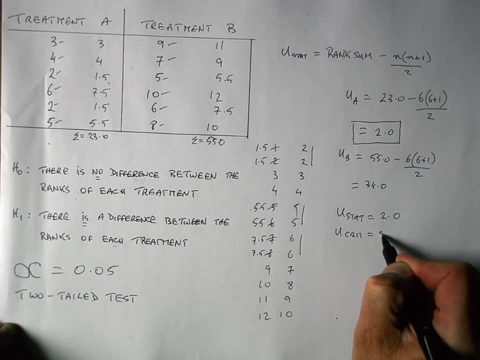 6 at alpha equal to 0.05.. So my U critical is 5.. So my U crit is equal to 5, 5.0.. So in this case, then, my result is that my U stat is less than my U crit at alpha equal. 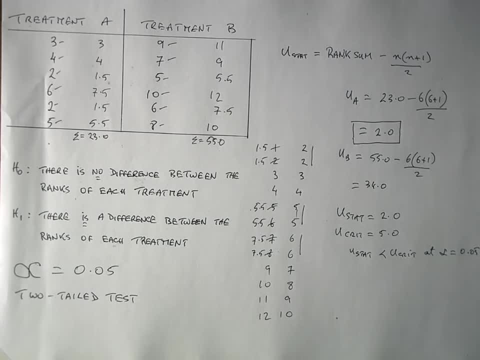 to 0.05.. To be statistically significant, our obtained U value of 2 here has to be equal to or less than the critical value of 5.. So this is different than other tests, don't forget, where the obtained value usually has to be equal to or greater than the critical. 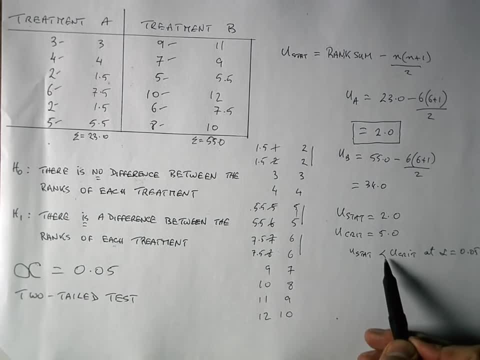 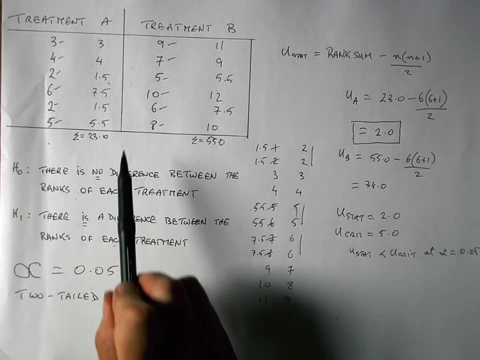 value. So our U statistic here is less than our U critical. Therefore we have found a difference. We can conclude that the difference we have found between the ratings over here for our two treatments is unlikely to have occurred by chance. So it looks as if the 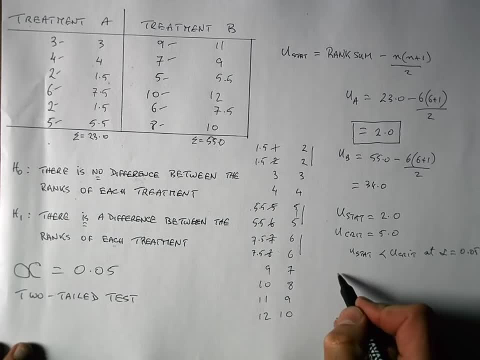 two treatments indeed do differ. So our decision here, then, is that we are going to reject the number of values in group 2.. So we can conclude that the difference between the two treatments is a null hypothesis, that there is no difference between the ranks of each. 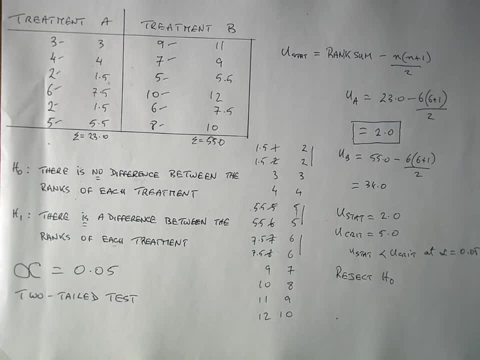 treatment in favor of the alternate hypothesis that there is a difference between the ranks of each treatment. We have concluded that there is a difference between the two treatments here using the Mann-Whitney U test. So that's how you calculate the Mann-Whitney U statistic. I hope you found this video useful. Thank you for your attention. 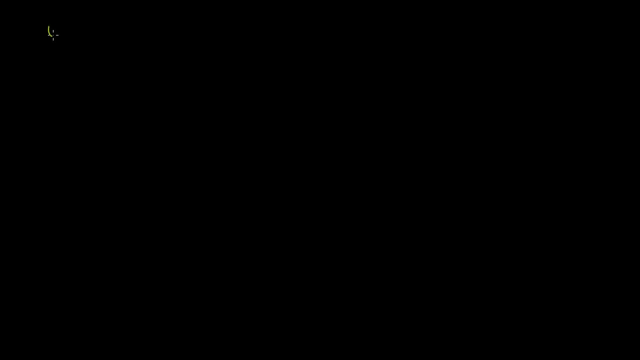 Let's graph ourselves some inequalities. So let's say I had the inequality. y is less than or equal to 4x plus 3.. On our xy-coordinate plane we want to show all of the x and y points that satisfy this condition right here.